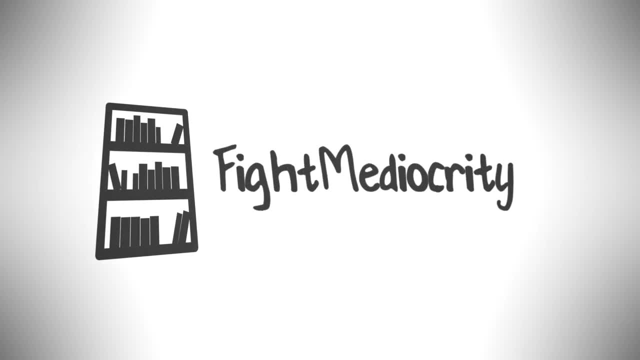 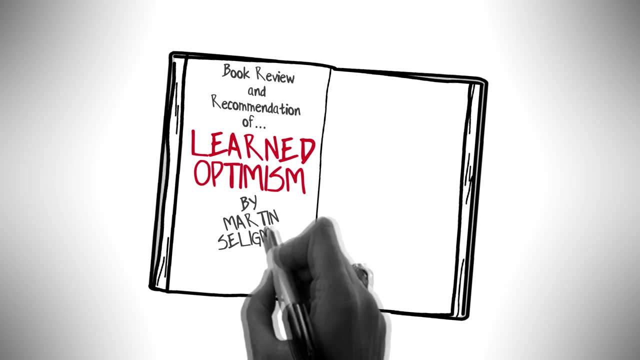 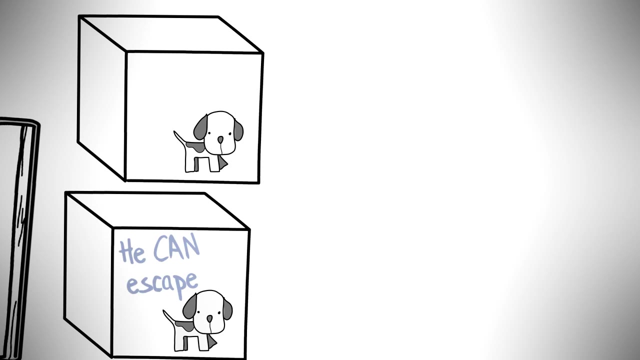 Imagine you take two dogs and put them in two different areas. You shock the first dog and you give him an option to escape. He tries to escape, he's successful and he gets away from the shocks. The second dog, however, you put in a place where, no matter what, he 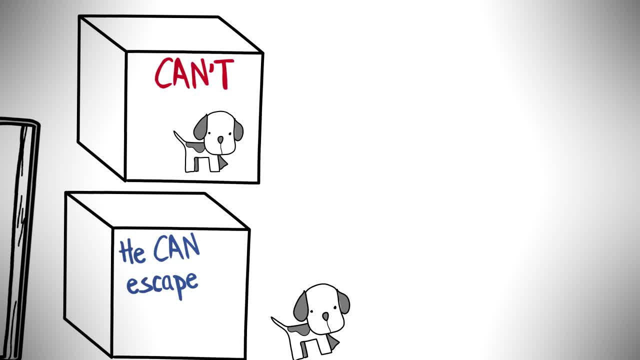 does? he cannot escape the shocks. He soon figures out that there's nothing he can do. He gives up and he'll just sit there and accept the shocks. Now you take these two dogs and put them in two new areas again, but this time they can both escape. The first dog who? 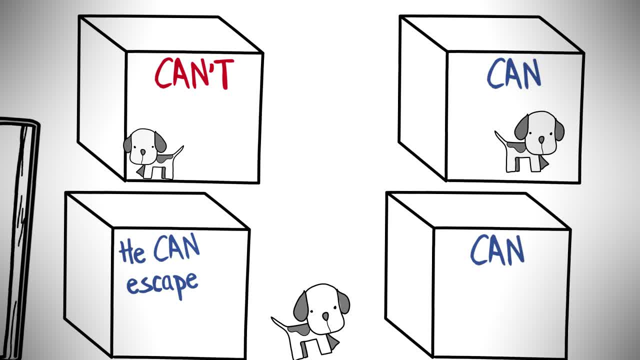 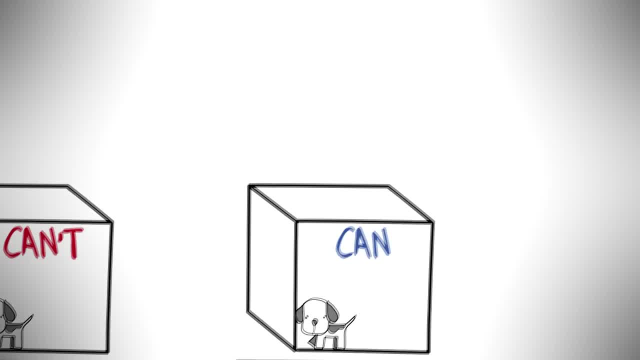 had learned that he was able to escape, will get out of there like usual, but the second dog will just lay there and accept the shocks, even though in this new environment he could just escape. This is what is known as learned helplessness, and you probably know people. 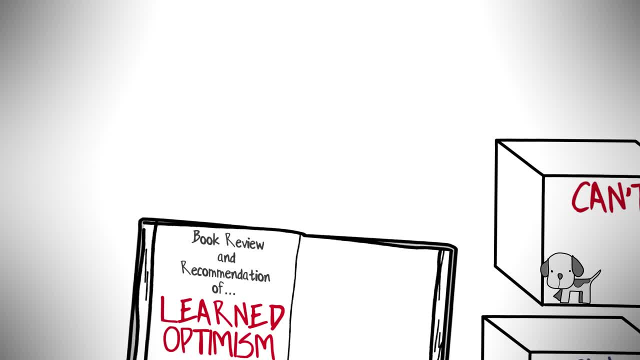 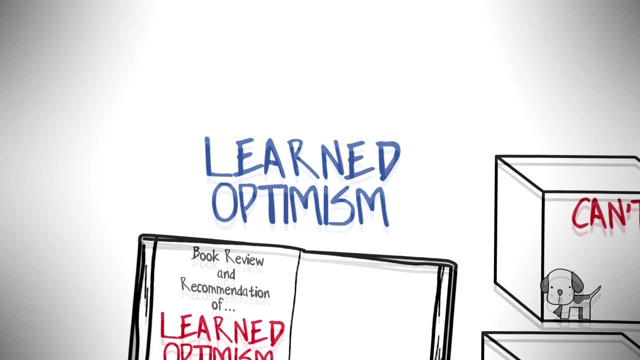 who act like the helpless dog. The opposite of this is learned optimism. Learned optimism is basically the idea that you can learn to be optimistic and positive and happy. You can cultivate these things, And this is exactly what Seligman was trying to do by running a workshop. The results of 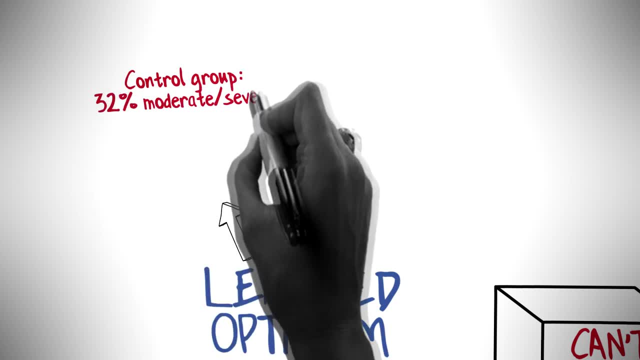 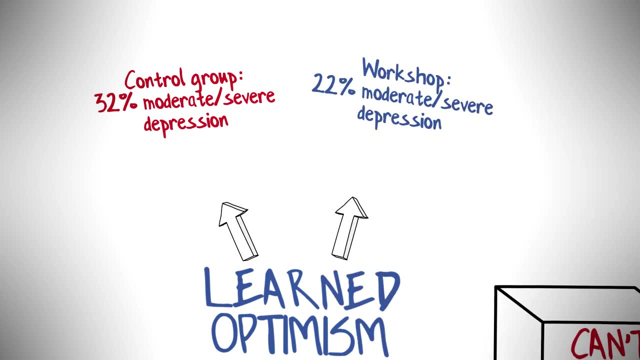 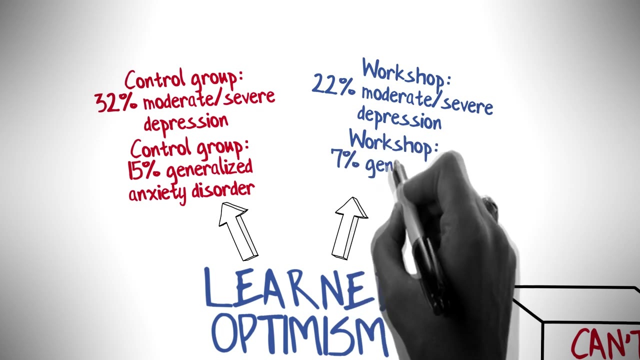 the workshop were promising. 32% of the students in the control group had a moderate to severe episode of depression, in contrast to 22% of the group that was in the workshop. Also, 15% of the controls had an episode of generalized anxiety disorder, versus only 7% of people. 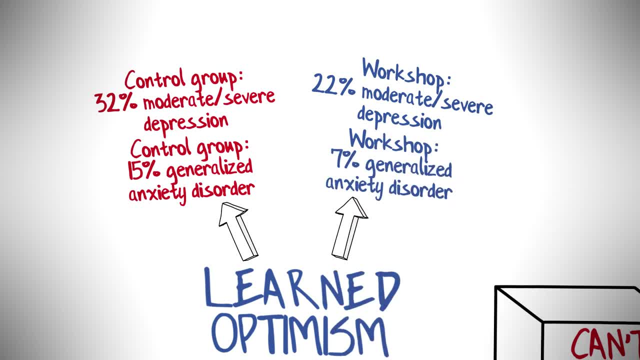 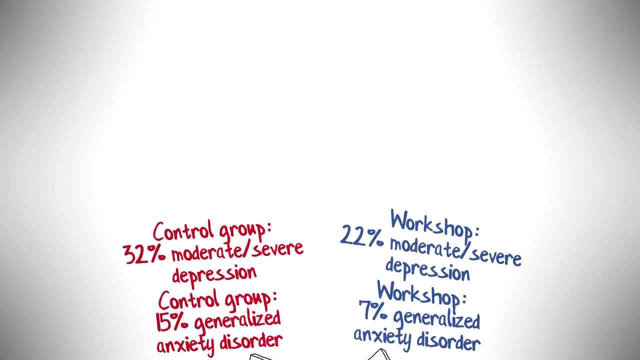 who took the workshop. They also found that it was the change from pessimism to optimism that caused the prevention of depression and anxiety. And these studies are great, but even when I look at my own life- happiness, positivity, optimism- these are the things that I've had to learn and that I have to keep cultivating. 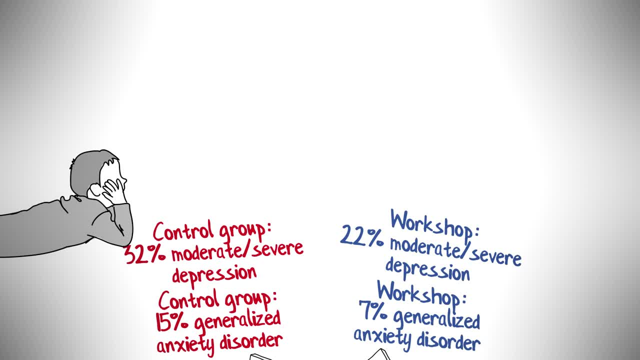 When I was a kid, I hated my life. I was constantly depressed and anxious. I was always worried. I was constantly depressed and anxious. I was constantly anxious. I was constantly depressed and anxious. I was constantly anxious. I was constantly depressed and anxious. I was constantly. 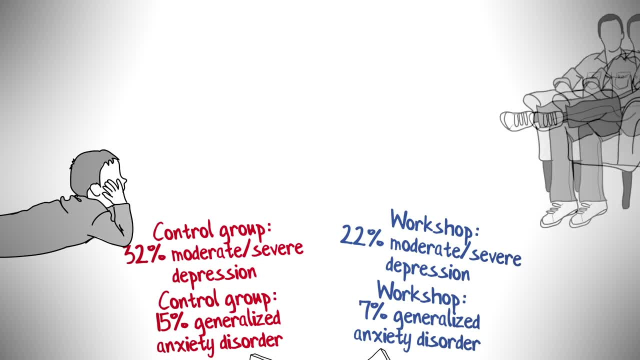 depressed and anxious. I was constantly depressed and anxious. I had suicidal thoughts for the majority of my childhood, but that's all gone now and my life just keeps getting better. But this is something that you need to put effort into. This is something that 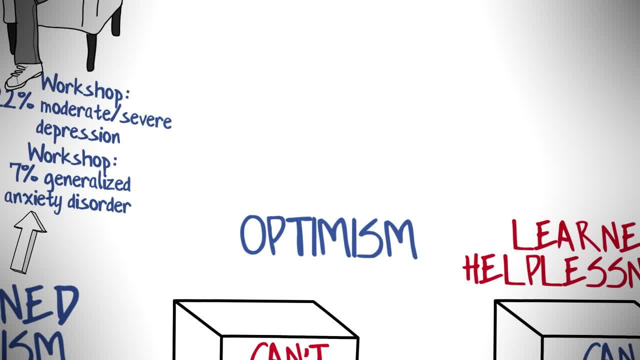 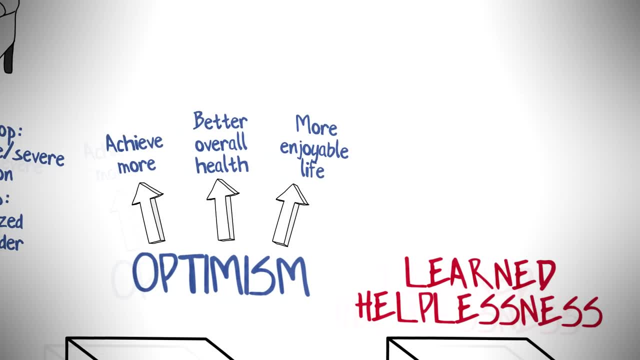 can be learned. So now let's look at the benefits of optimism. Optimists, on average, achieve more, have better overall health and just lead a more enjoyable life. Pessimists, on the other hand, are more likely to give up, are more likely to suffer from depression and just lead a not really 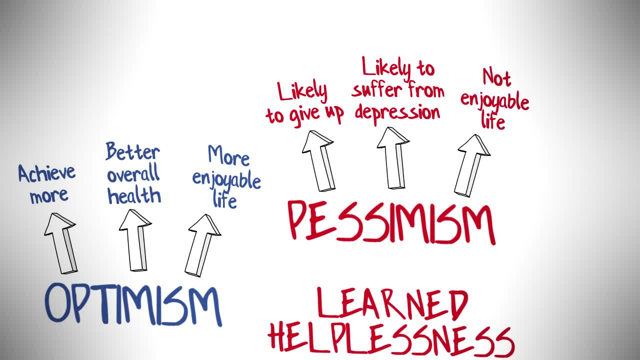 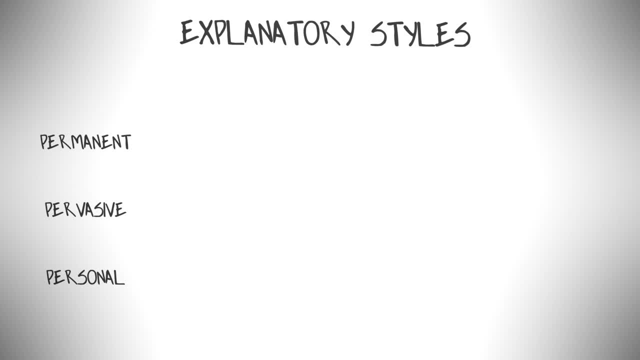 enjoyable life comes from their explanatory styles about whether things are permanent, pervasive and personal. So let's say, you walk up to a girl and you just get humiliated and rejected. If you're a pessimist, you'll think that it's. 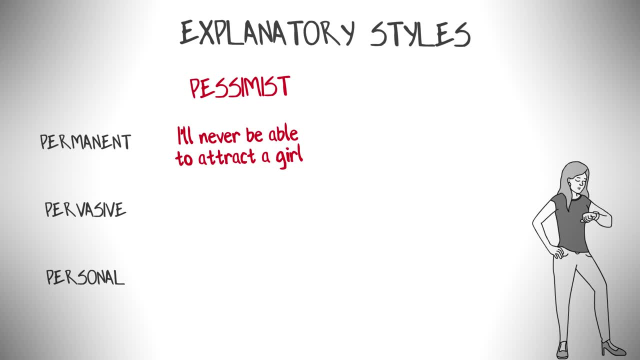 permanent, I'll never be able to attract a girl. If you're an optimist, you'll think that it isn't permanent. There are going to be plenty of girls who like me. If you're a pessimist, you'll think that it's pervasive. I'm just not an. 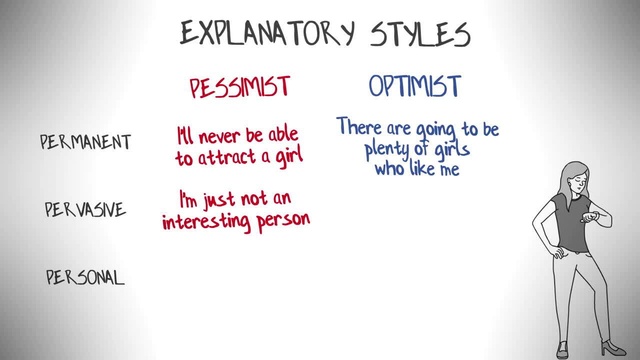 interesting person. If you're an optimist, you'll think that it isn't pervasive. It was just one isolated situation. It doesn't mean that I'm not interesting. If you're a pessimist, you'll think that it's personal. I'm ugly, Of course she's. 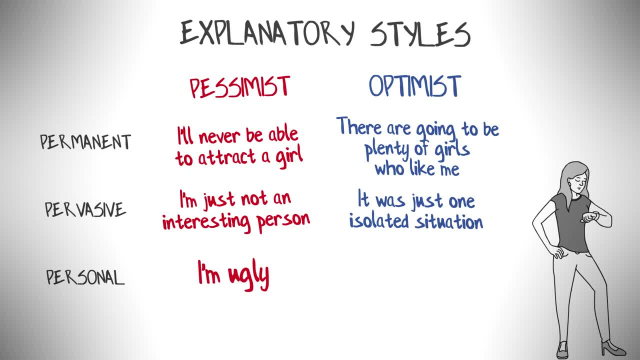 going to humiliate me. If you're an optimist, you'll think that it isn't personal. Well, she might have been in a bad mood, And I've seen this so many times. If you have a pessimistic explanatory style, you're going to have 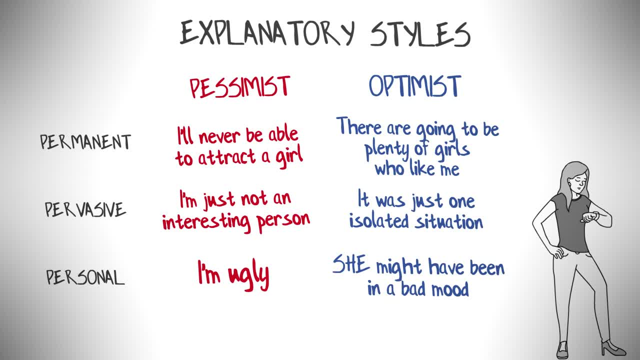 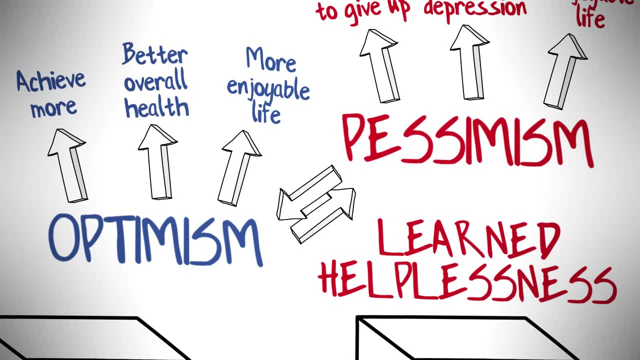 your soul crushed. Every single friend I've had who was good with women always had an optimistic explanatory style, So optimism is much more helpful to you than pessimism. but you also need balance. Just like with everything else, you need balance, Otherwise you can get really. 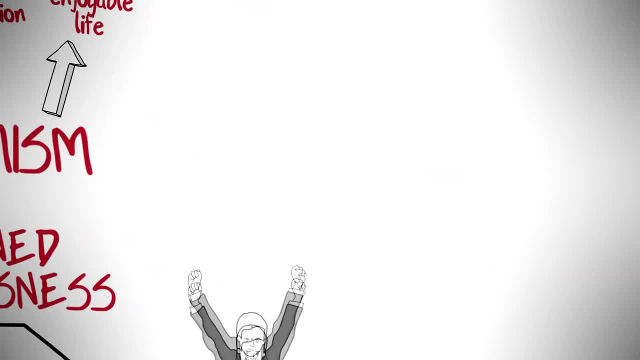 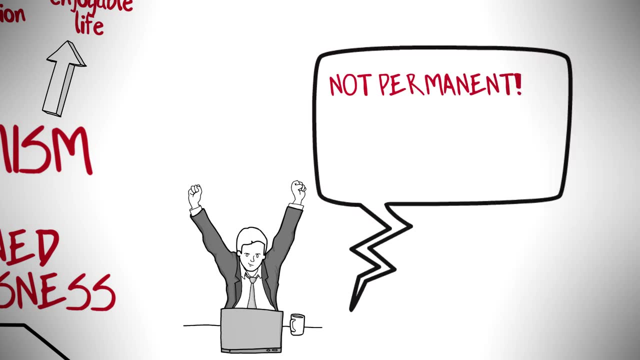 delusional and actually end up hurting yourself. Imagine if you have a really bad business idea and you're just a naive optimist. The business isn't going anywhere, but you say, well, this isn't permanent And you keep wasting resources on a stupid idea you've put in six months. 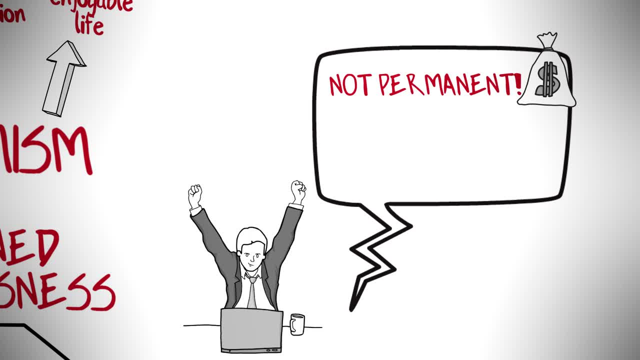 months already and it hasn't gone anywhere and you say, well, it's just this part of the project that's slow, but the project as a whole is amazing. Or you try to get support and no one wants to go along with your terrible idea and you say, well, they were probably just in a bad mood today.